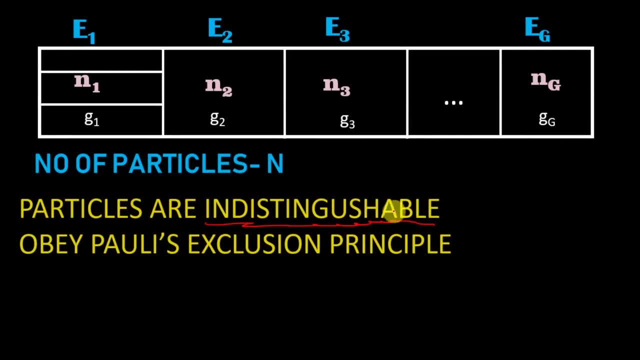 is not been cancellated and the particles are indistinguishable as they are in the Bose Einstein stat. but in this the difference is they obey Pauli's exclusion principle, and this makes this thing really easy to find. because of this, like one particle can go in one energy level. 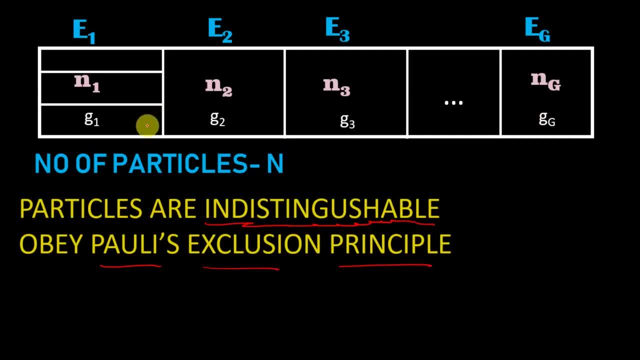 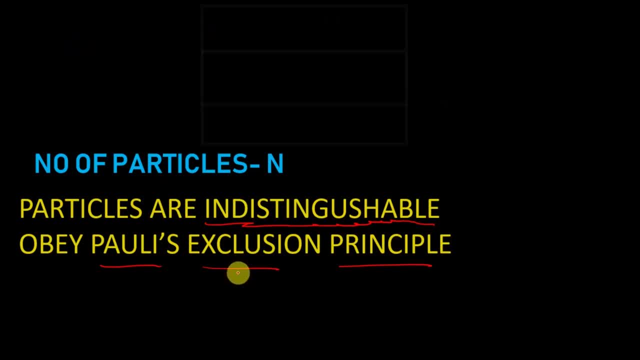 so this makes finding this thermodynamic probability really easy, easier than Bose Einstein stat and very easy than Maxwell Boltzmann stat. So they obey Pauli's exclusion principle. So if we have like three energy level and three particles, like one can go in here, the other should go in other energy level. no two particle can fill the same. 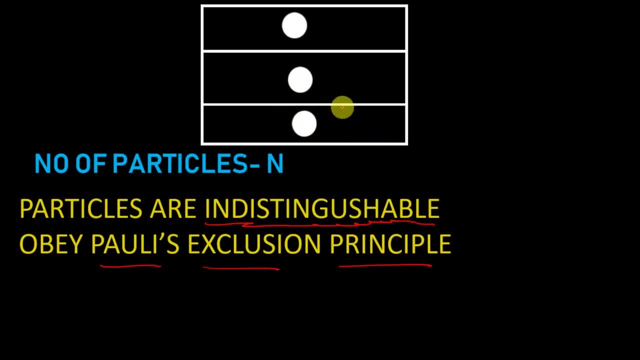 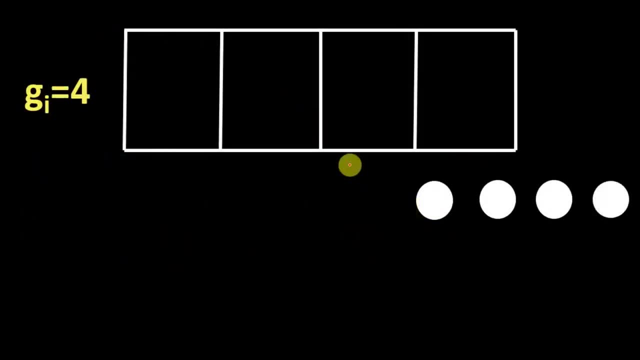 energy level. So one specific energy state will have only one particle. this is what Pauli's exclusion principle is. Now, to find this, let us assume this simple case: we have one energy level which have a degeneracy of four, like there are four different partitions in this main energy. 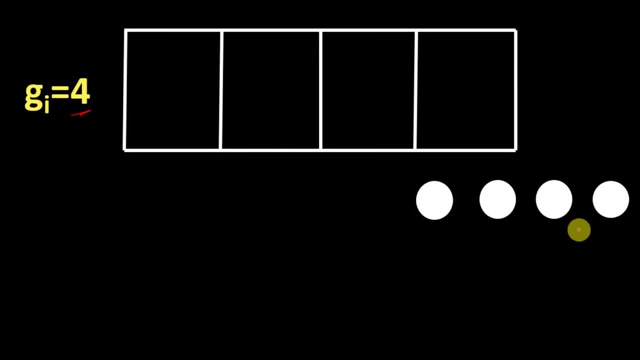 level and we need to distribute like four particles in here. Now if somehow we are able to find in how many ways these particles can arrange themselves in this one main energy level, then we will automatically get it for all the energy levels and then we will multiply it as we have. 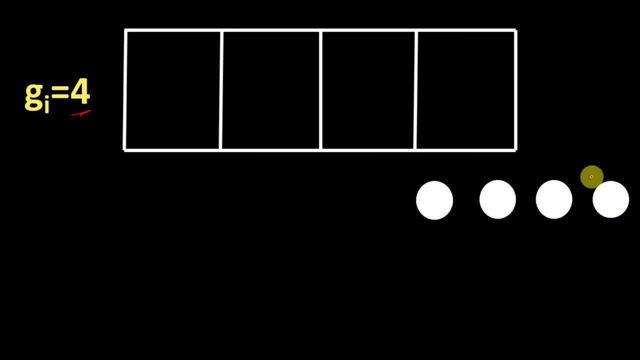 done in Bose Einstein's stat. So we just need to find in how many ways these particles, these Ni particles, can arrange themselves in these Gi sub levels of this main energy level. So we need to do this Now. see this: this obeys the Pauli's exclusion principle. So for the first choice, we 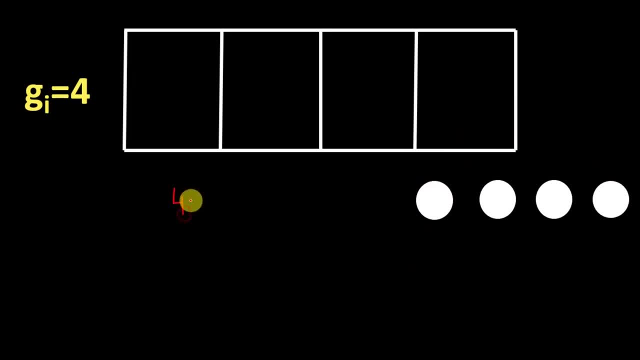 have this four Particles. so we have like four choices first. then we will like fill one of them in here. now we have three choices, now like we have two choices, now we have one choice and now we have no choice. So this is the number of ways in which these particles can be picked to fill this energy level. So the number. 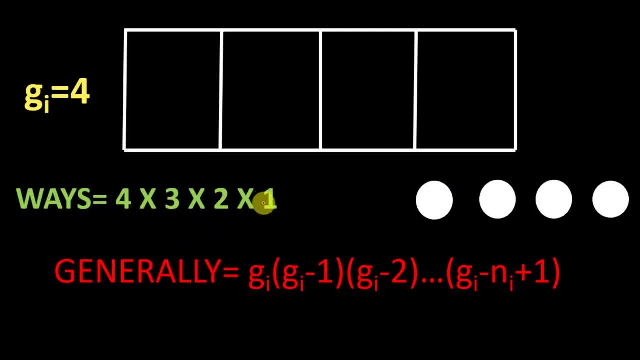 of ways are like four multiplied by three, multiplied by two, multiplied by one. Now, generally it is this: four is Gi. so Gi Gi minus one, Gi minus two and so on, to see this Gi minus Ni plus one. So look at it in here, for example, this is Gi four minus four. so ending is an in one. but if you have, 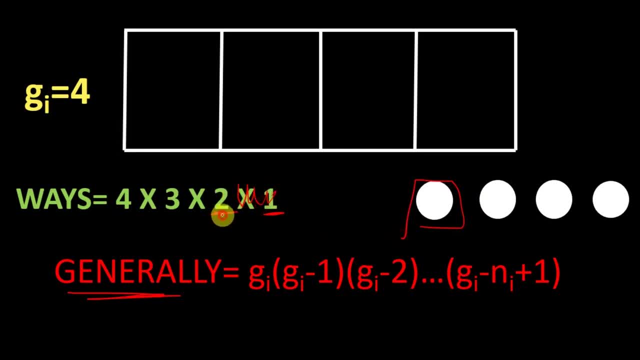 like three particles. then this ending is here in two, so Gi minus Ni, which will be one, one plus one is two, so this is a general formula for this one. now, this is basically the number of ways in which these particles can fill in here, but we need the final result in factorial way, so we will like convert this thing in factorial. 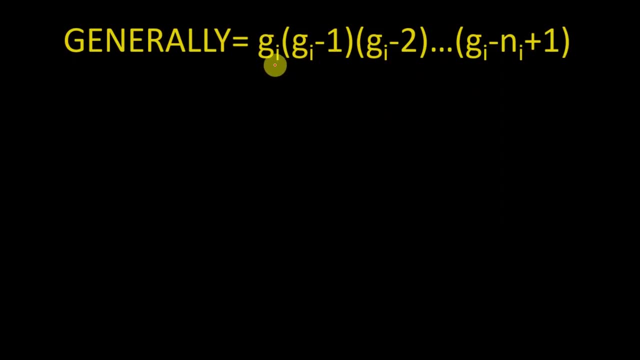 so we have this. now. what we'll do is this: see this: this is gi gi minus 1, gi minus 2, and so on to gi minus ni plus 1. now, if we multiply it by gi minus ni, okay, that means gi minus ni plus 1. 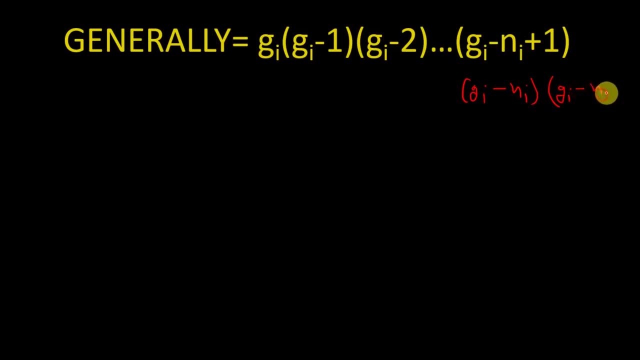 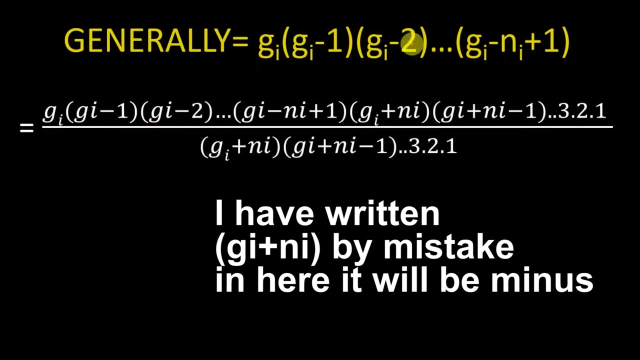 minus 1, and then gi minus ni minus 1, and so on to 3, 2, 1. what is this? this is gi, factorial, so we have multiplied it. we will divide this 2 to not change this expression. so we have this thing in here, that is, this part multiplied by that part and divided by that part. now, this above thing. 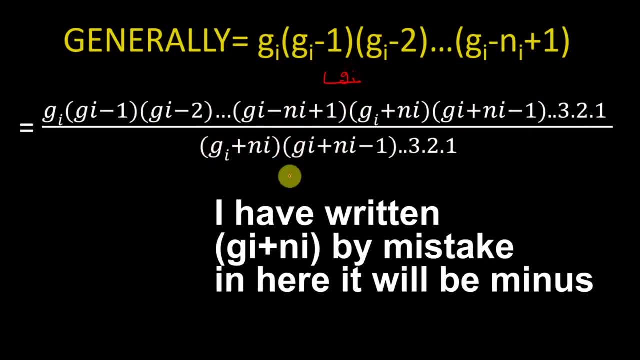 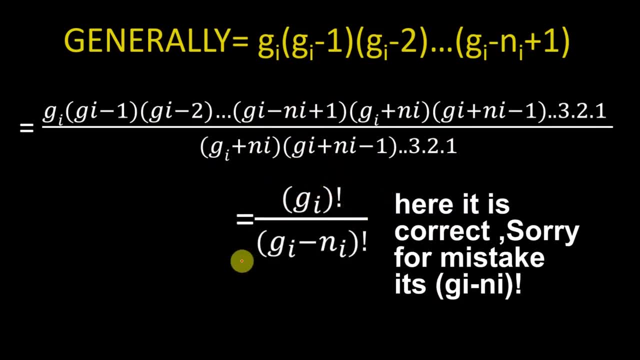 is gi factorial and this down thing in here is gi plus ni factorial. okay, so we have this thing in here: this is gi factorial and this is gi minus ni factorial. but see this in the above way that we did, like we did: 4, 3, 2, 1, what we did is this: the self-changing 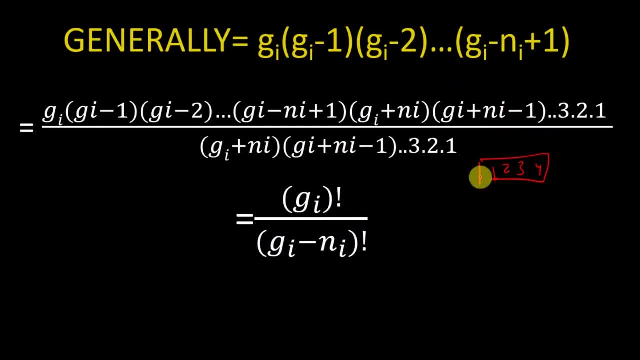 of those particles will be counted automatically in here. so to solve that, what we will do is this: as we have done in the permutation combination video: we can change from a permutation to a combination if you don't want to like count the ways combination video: we can change from a permutation to a combination if you don't want to like count. 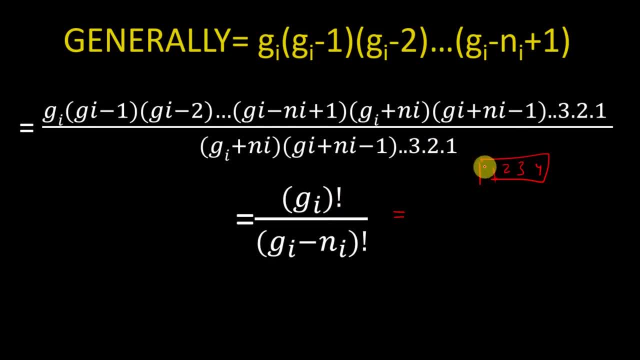 the ways from the particles changing their position, like switching their position. then we will divide this whole thing by ni factorial the number of particles, like n things can arrange themselves in n factorial ways. so that is what we will apply here. we will divide that n factorial in here. so divide it by. 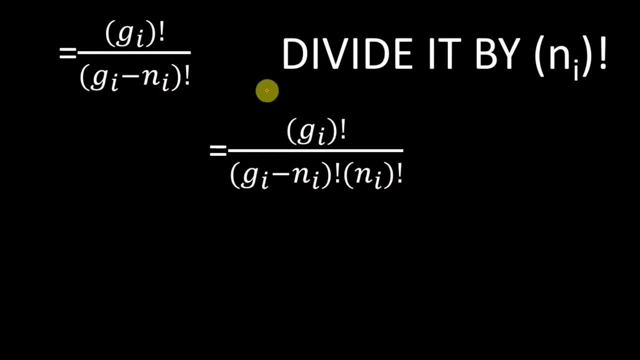 ni factorial. divide this thing by ni factorial. so this is basically the number of ways in which those indistinguishable particles can arrange themselves in that energy level. so now, generally for fermi dirac, stat 6, we will multiply this thing for all the energy level.